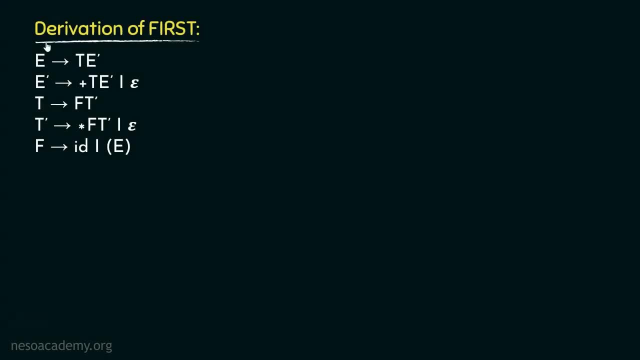 of the first and follow functions. Let's begin with the derivation of first. Now, during the derivation of first, it's always a good idea to start with the last non-terminal, And the reason behind that is- notice this: we are dealing with top-down parsers without 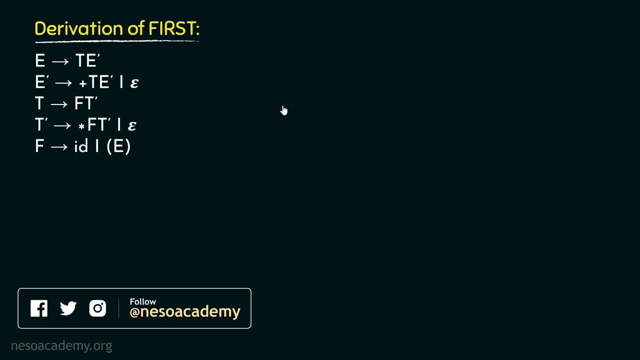 backtracking. Now, parsers can't really handle ambiguity, except for operator precedence parser. So definitely the grammar that we will be dealing with will be unambiguous Thereafter. L1 parser is a top-down parser. Now, top-down parsers can't handle ambiguity. 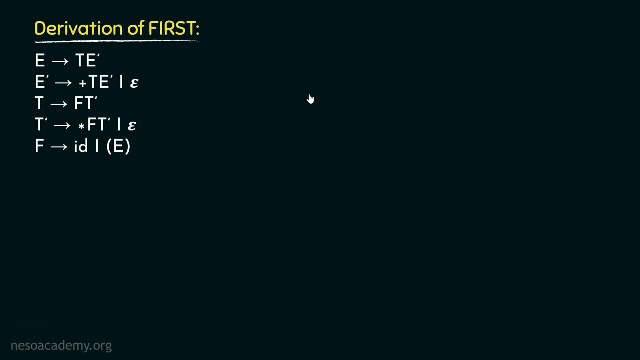 They can't deal with left recursions. If left recursions are there, there is a possibility of getting into infinite loops. Therefore this grammar is supposed to be right: recursive, which, if you notice carefully, is true as well. Observe here the non-terminal e dash. 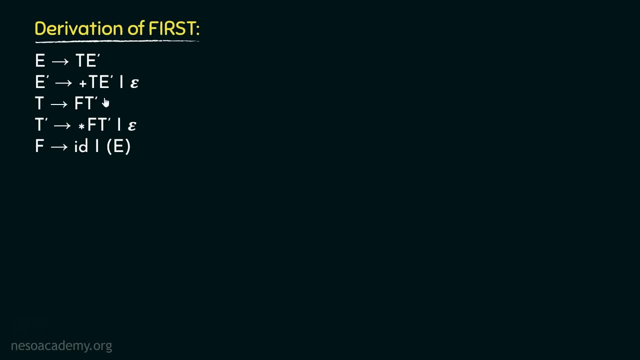 is also the rightmost non-terminal on the right hand side. Then again, for this non-terminal t dash on the right hand side, the same non-terminal t dash is the rightmost element. Also, these types of parsers can't deal with non-determinism. That means the grammars. 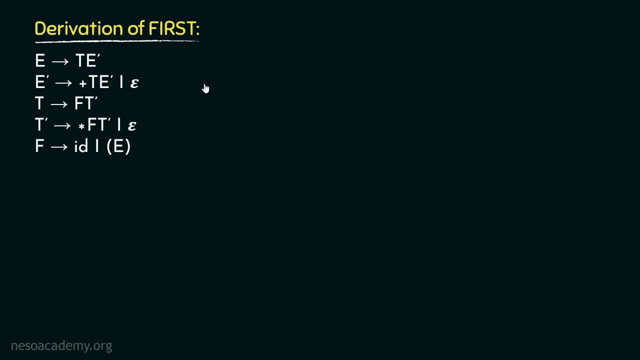 will be free from any type of non-determinism And for these kinds of grammars, the list of the production rules always begin with the start symbol And the list follows in such a way that the non-terminals at the bottom of the list are more likely to provide us with the terminal symbols directly. 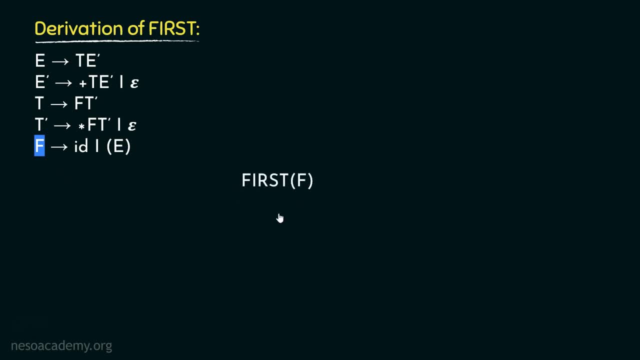 So let's take a look at the first of f. Now, coming to the first of f, as you can observe the production rules f can be rewritten as either id or this. So the first of f is going to have the terminal symbol id at first. Now, considering this production rule, we 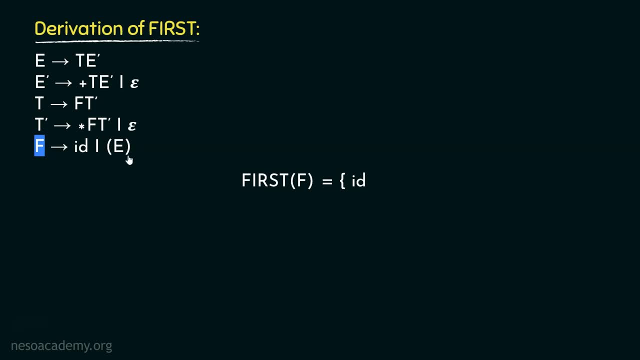 have open parenthesis e, followed by close parenthesis, And here these two are terminal symbols. So, considering this production rule, we can state: in first of f, alongside the first of t, we will also have the terminal symbol open parenthesis. So let's analyze. 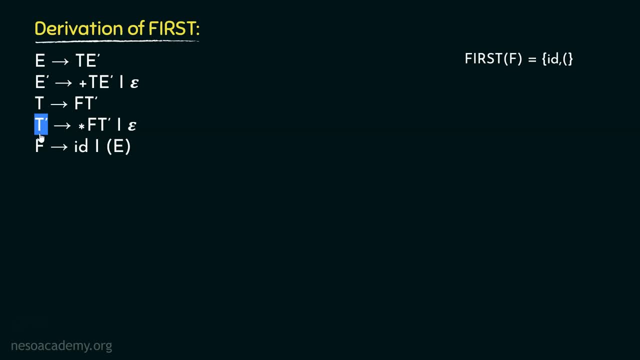 that. Now let's move on to the next non-terminal, that is t dash. So the first of t dash is going to include the symbol star. following this particular production rule, T dash can be rewritten as star, followed by capital F, followed by t dash. And here the first terminal. 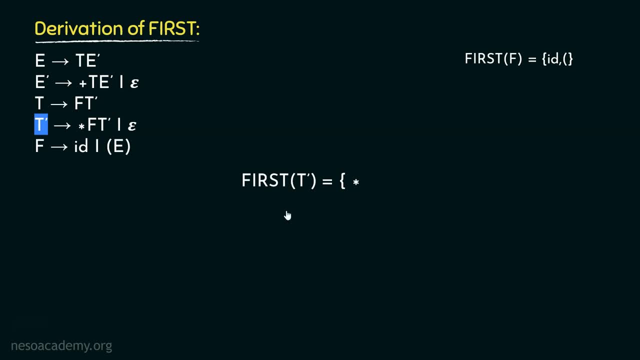 is the star. Therefore we are keeping star as the first of t dash. Now let's see if we can get the first of t dash. So the first of t dash has another production rule, that is, t dash can be rewritten as epsilon. Therefore t dash can also derive. 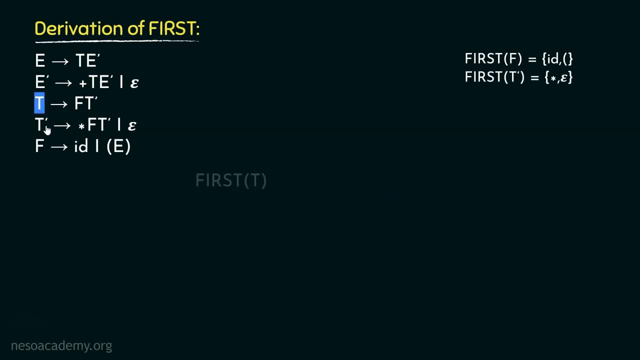 epsilon. So in first of t dash we will also include the symbol epsilon. Let's analyze that too. Coming to the next non-terminal, that is t. So the first of t can be determined from this production rule. t can be rewritten as capital F, followed by capital t dash. Now, 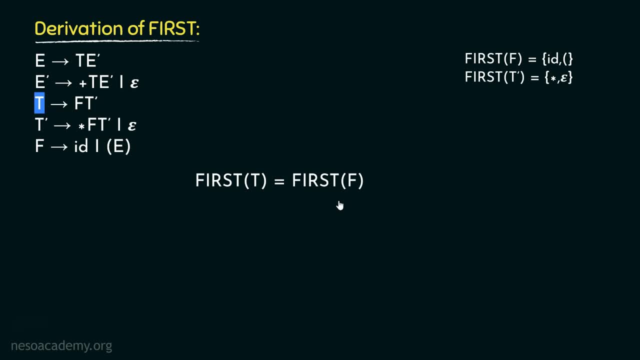 t dash can be rewritten as capital E dash, But t dash can be rewritten as capital E dash. So let's see how it is going to be. So the first of t will include the first of F, That is, all the symbols that F derives will also follow in the derivation process from t right. 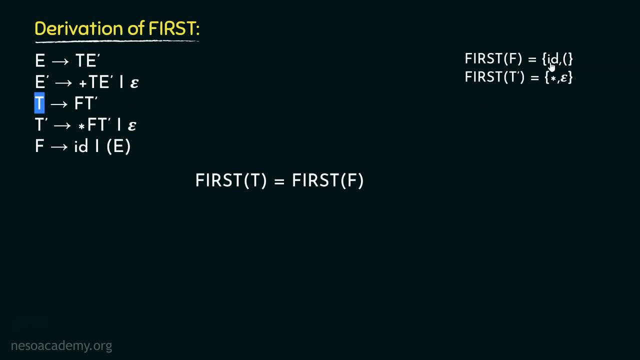 Now we already have enlisted first of F, which is id and the open parenthesis. Therefore the first of t will also include these two terminal symbols. So let's analyze that too. Coming to the next non-terminal, that is E dash, Let's determine the first of E dash. 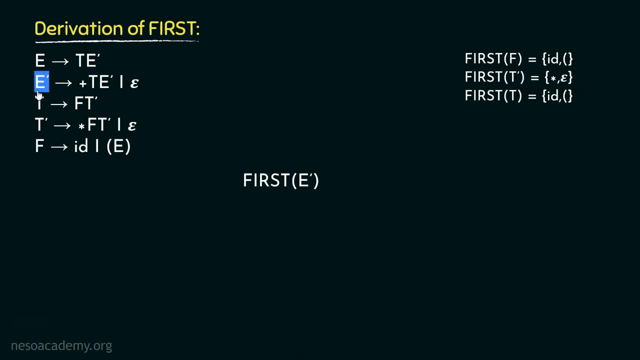 now E dash have two different production rules. One is E dash can be written as plus, followed by capital T, followed by capital E dash, And the other one is E dash can be written as epsilon. Now from this one we can say: this is the terminal symbol. So in first of E dash we will have plus, And from 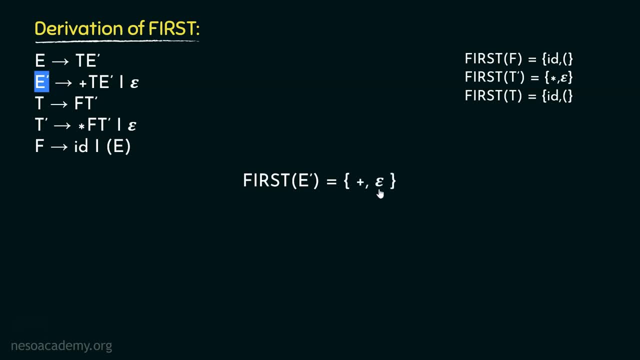 the other production rule, we will include the epsilon symbol. So the first of E dash will have plus and epsilon. Now, finally, we have the start symbol E. Let's find out. the first of E, Observe E can be rewritten as capital T, followed by E dash. Now, here also, we don't really have any. 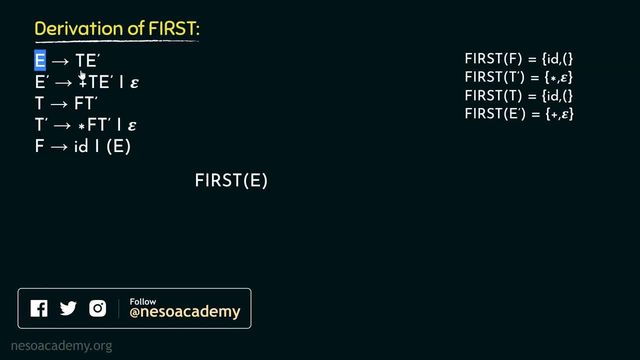 terminal symbols right away. However, the symbols generated by T will also follow in the derivation from E. that is the start symbol. Therefore, the first of E will include the first of T, which are the terminal symbols, id and open parenthesis. Let's enlist that too. Now we have found out the firsts of all the. 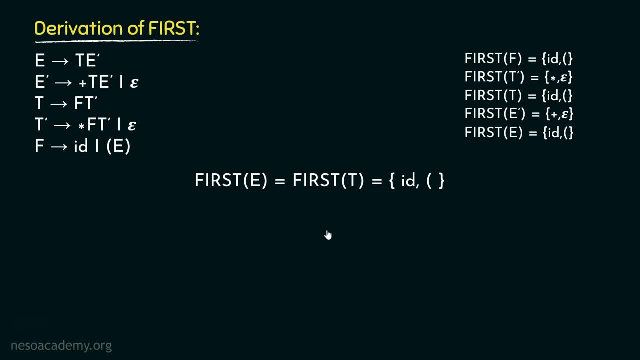 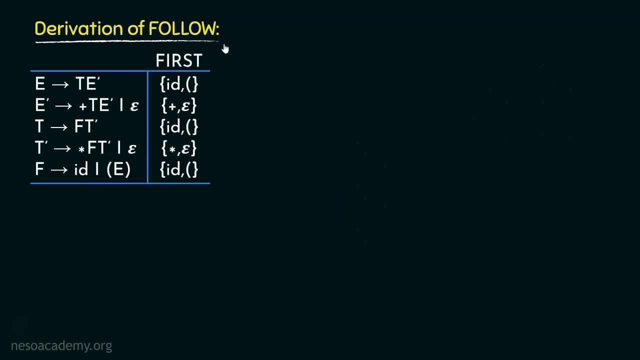 non-terminals involved in that grammar. However, we enlisted them in reverse order, So let's correct that order. So these are all the firsts of all the respective non-terminals involved in this grammar. Let's now proceed with the derivation of: follows: Now the reason behind beginning with the derivation: 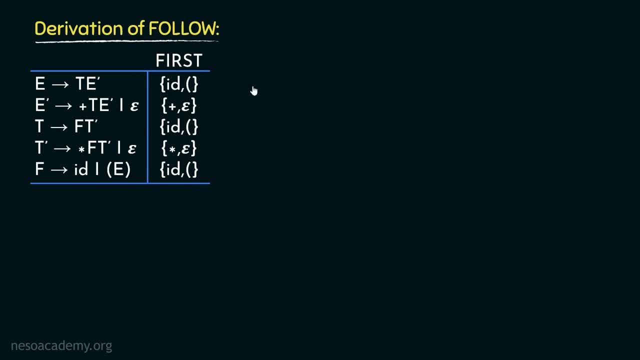 of first is that these are going to be the firsts of all the non-terminals involved in this grammar, So they are going to be very helpful for the derivation of follows. So let's start off with follows now. Now, coming to the derivation of follow, we can always start with the start symbol. 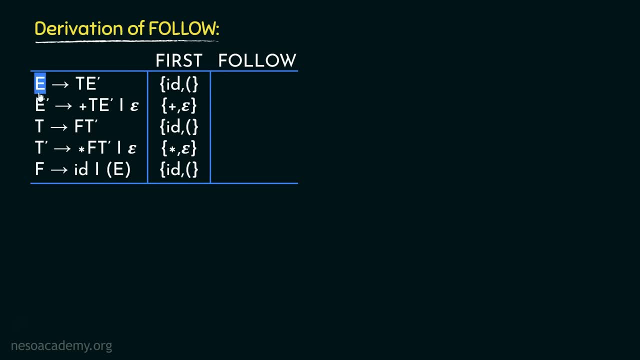 There is no harm in it. Now lets find out the follow of E. Now, before we dive straight into this, I'd like to provide an illustration. Say, we have a production like this: s can be rewritten as a, b, followed by capital C, And clearly this is the start symbol. Now, in the buffer, when 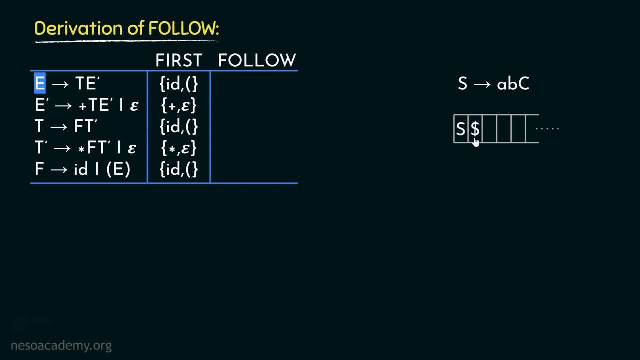 When S will be stored, it will have the dollar symbol following it And eventually, when S will derive, this ie A, B, followed by capital C, in that case this dollar symbol will also follow this non-terminal C. So always remember for start symbol in. 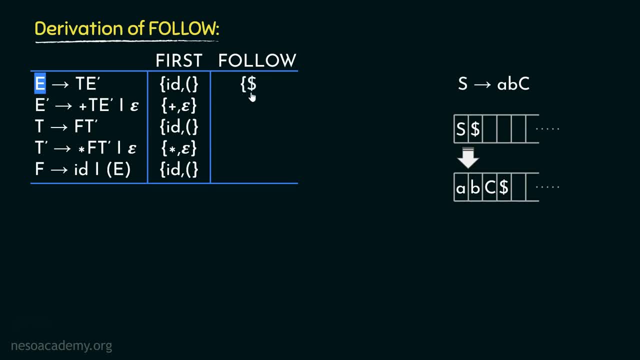 the follow set, the dollar symbol will always be there. Now, apart from this, E also appears in this particular production rule where this non-terminal E is being followed by the terminal symbol, close parenthesis. So in the follow of E, alongside this dollar symbol, we are also going to have the terminal. 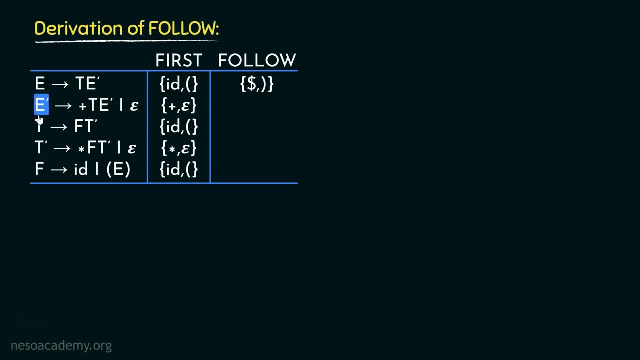 symbol- close parenthesis. Let's move on to the next symbol now. So we are going to determine the follow of E' Now. observe: E' appears in these two production rules, Now in this one it has nothing to follow. Therefore, whatever will follow E will also follow E'. 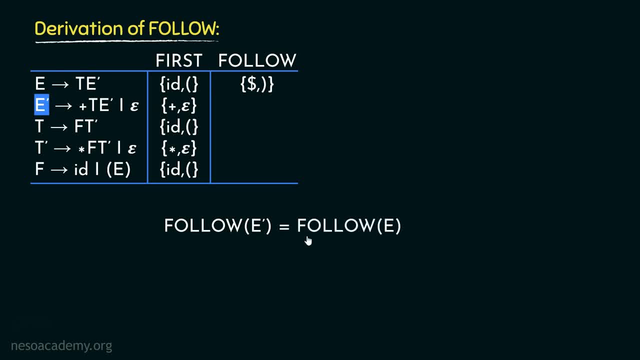 So the follow of E' will include the follow of E, And in follow of E we have the symbols dollar and close parenthesis, So let's include that Now. apart from this, E' also appears in this particular production rule. Considering this, here, the follow of E' is actually is the follow of E', whereas this: 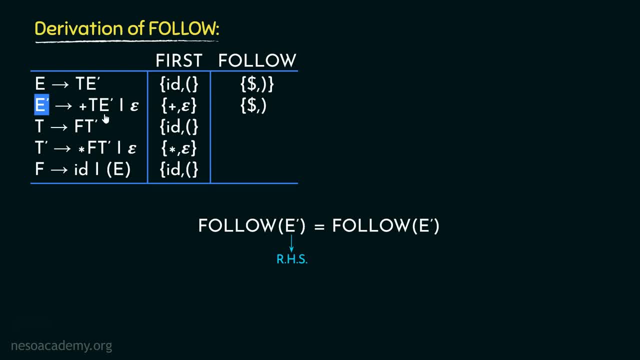 E' is the right hand side. ie this E'. On the other hand, this one is the E' of the left hand side, ie this E'. So, basically, we will wrap it up in here, only Now coming to the next symbol, that is, non-terminal T. 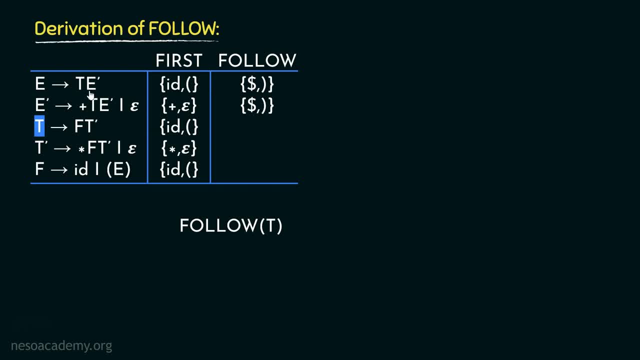 Now, in order to determine the follow of T, we will have to consider these two production rules, because these two are the places where T appears on the right hand side, And in both the cases, T is being followed by E' Therefore, the follow of T will include the first of E'. 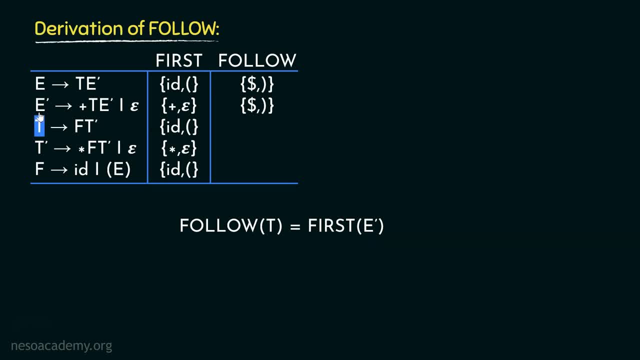 That is all the symbols which can be generated from E' will have to be considered now. Now in first of E' we have the symbols plus and epsilon Now in this set. this is a terminal symbol, So we can definitely include that. 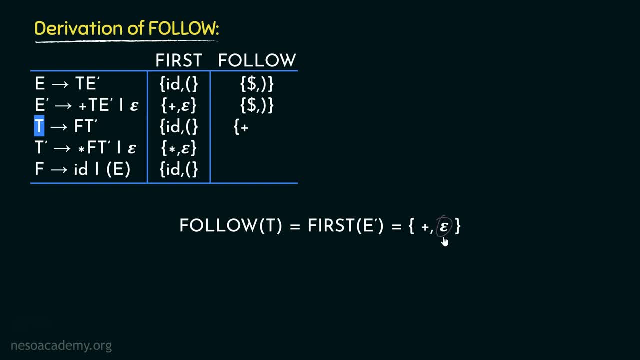 However, in case E' derives epsilon, there can be three cases. The first one, the following terminal symbol will be selected as follow: Now, in these two cases, T is not being followed by any terminal symbol, So we can definitely include that. 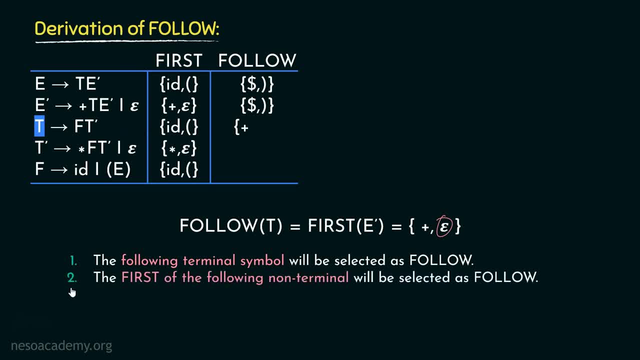 So let's move on to the next one. The first of the following non-terminal will be selected as follow: So in case E' derives epsilon, we also don't have any non-terminals which follows T in these two production rules. So let's observe the third one. 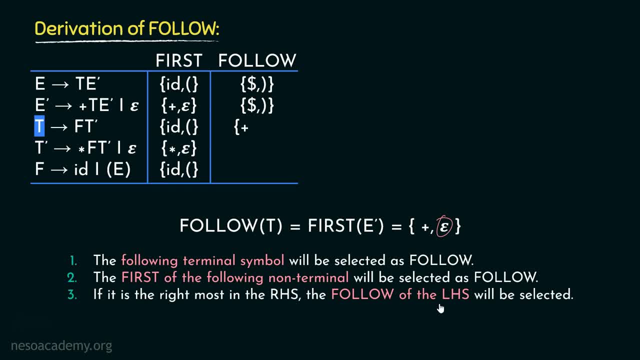 If it is the rightmost in the right hand side, the follow of the left hand side will be selected. Now notice: if in both the production rules E' derives epsilon, in that case T is being followed by the rightmost symbol in the right hand side. 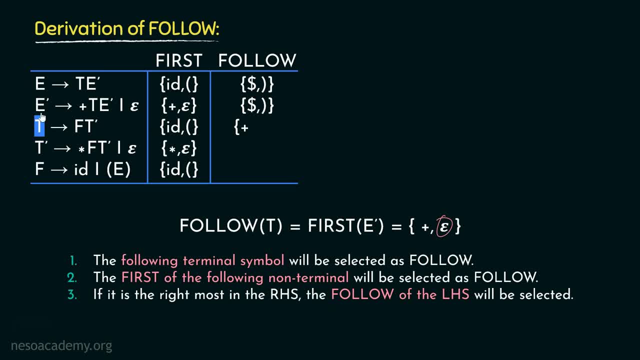 In that case we are going to select the follow of the left hand side. Now observe the follow of E and E' It is the same. So alongside plus, in the follow of T we will also include the dollar symbol and the close parenthesis. 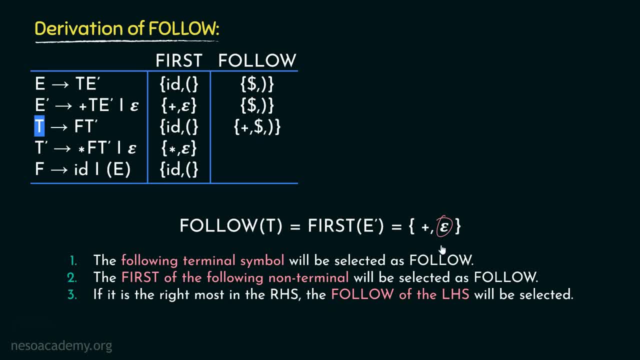 Do remember: the first of any symbol can include epsilon. however, follow of any non-terminal will never include epsilon. Let's now move on to the next non-terminal, that is T'. Now the follow of T' can be determined from these two production rules. as T' appears. 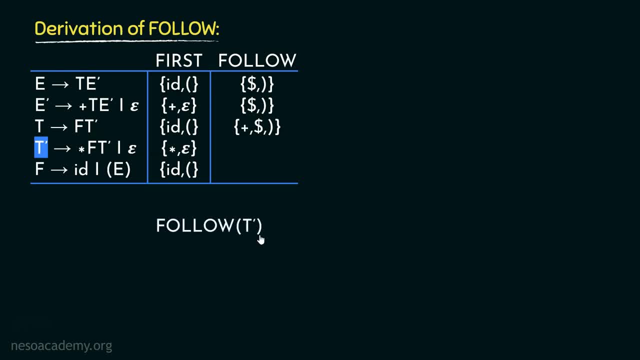 in the right hand side of these two. So the follow of T' according to this particular one will include the elements from follow of T And for this one it is redundant. So from this one we can get plus dollar and close parenthesis.